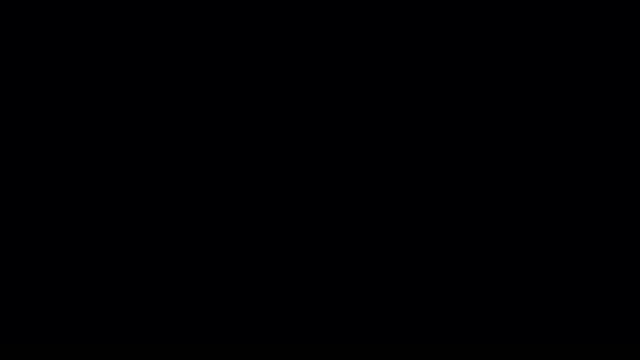 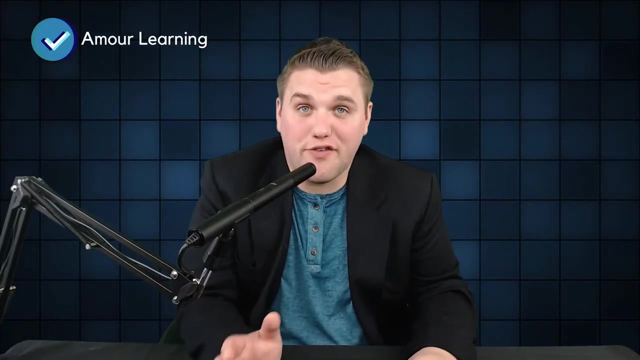 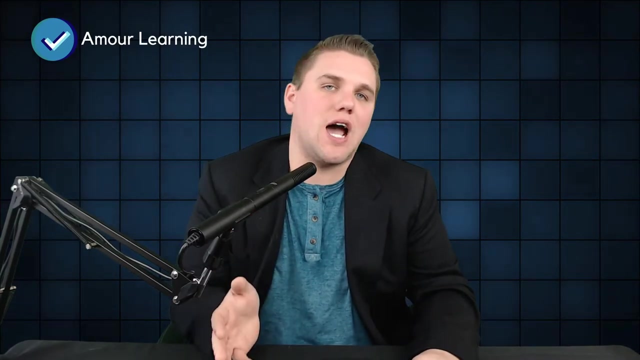 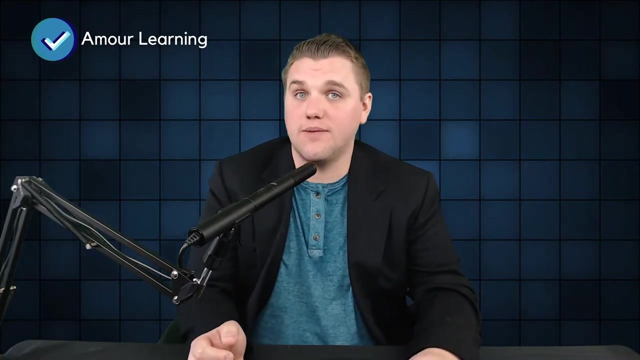 Recursively defined functions are often easier to create from a real-world problem, because they describe how the values of the functions are changing. However, this comes with a price. It is harder to calculate the image of a single input, since you need to know the images of. 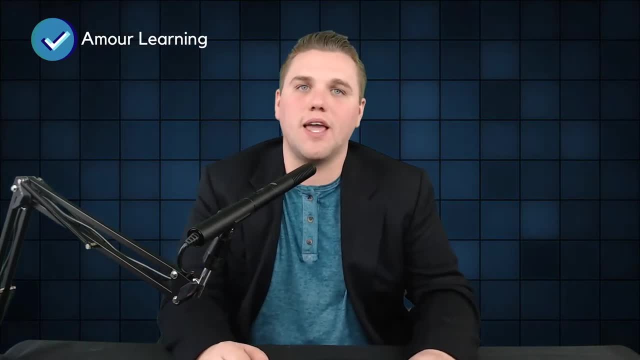 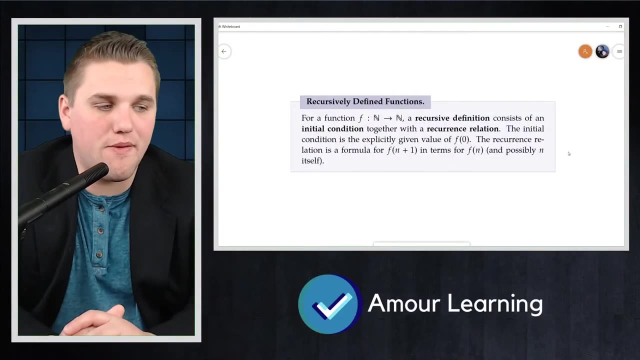 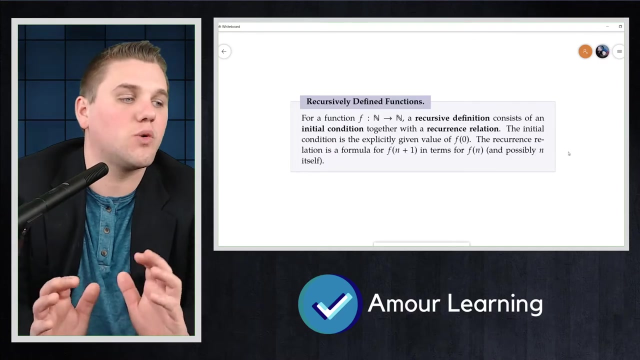 all the previous elements in the domain. Let's take a look at the definition of a recursive function. For a function f from the natural numbers to the natural numbers, a recursive definition consists of an initial condition together with a recurrence relation. The initial condition is the explicitly given value of. 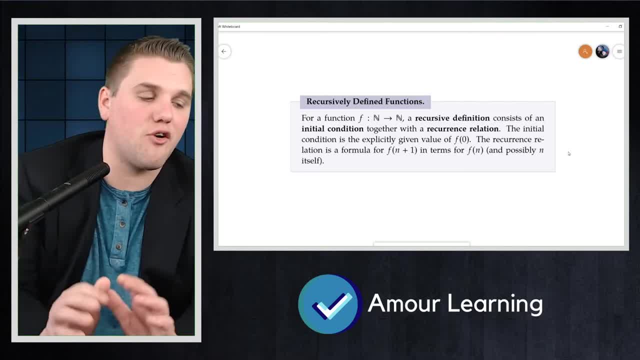 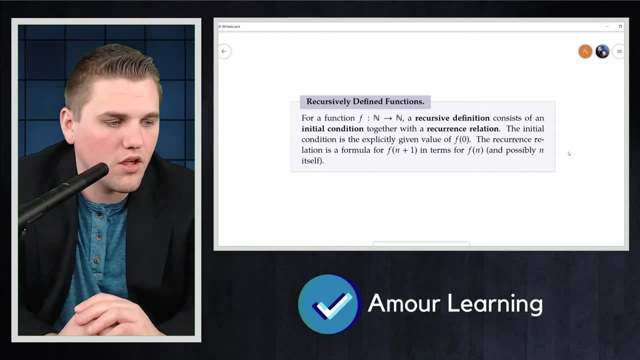 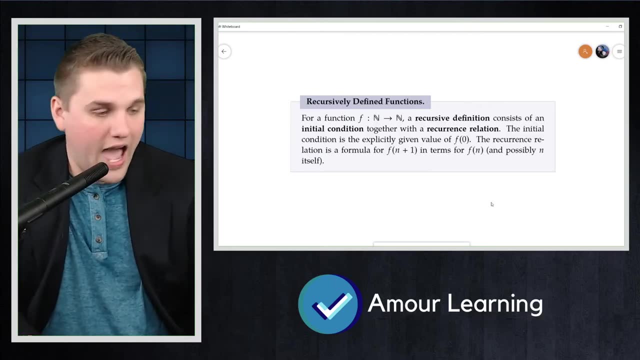 f. The recurrence relation is the formula for f in terms of f and possibly n itself. So let's go through some examples together so that we can understand exactly what this means. I have an example here. actually, Let me scroll down here so we can go through this. 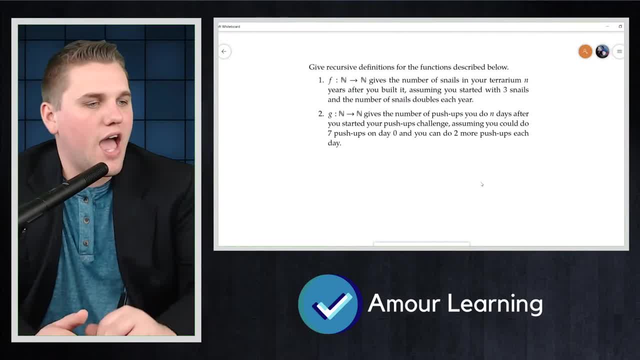 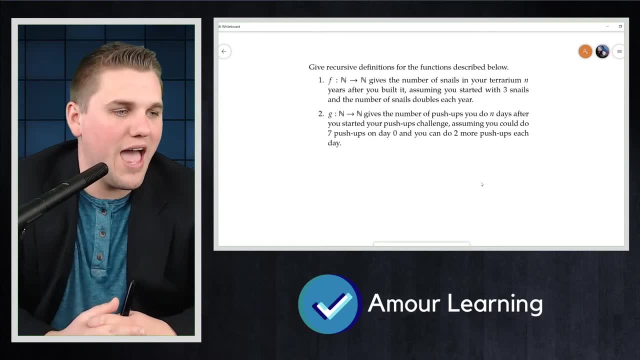 Give recursive definitions for the functions described below. f- sends from the natural numbers to the natural numbers. gives the number of snails in your terrarium n years after you built it, assuming you started with three snails and the number of snails doubles each year. 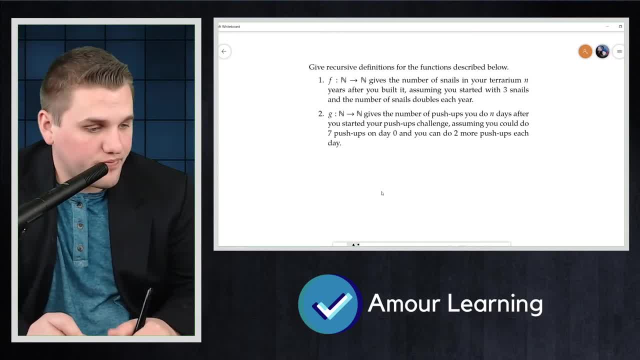 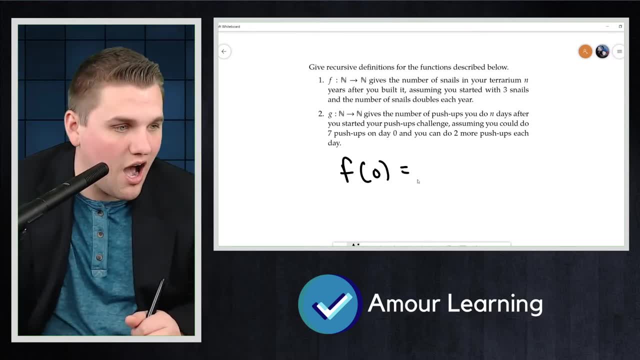 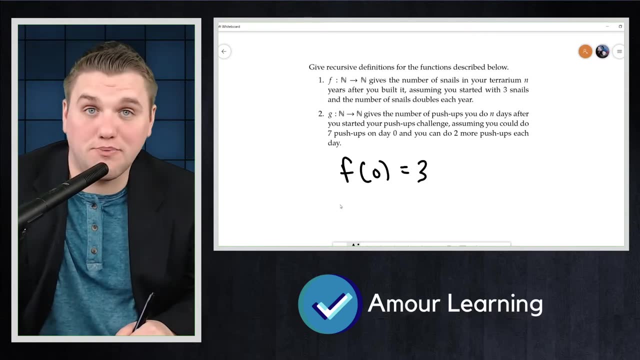 The fist thing we need is the initial condition: brauch & exist. ptlo, attr $, id. How many snails do you start off with? 3,, okay, I am catching up Next moment. This can be something I just raised earlier. For a rule, a state number equals 3 units. 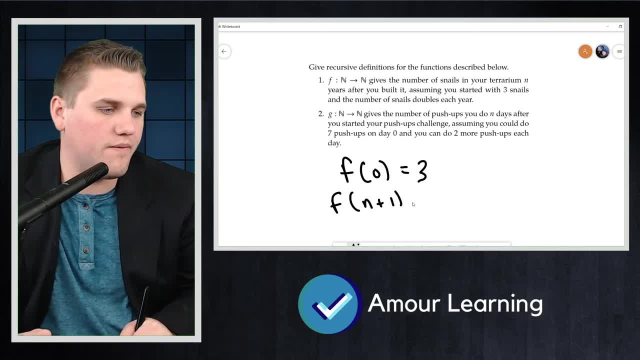 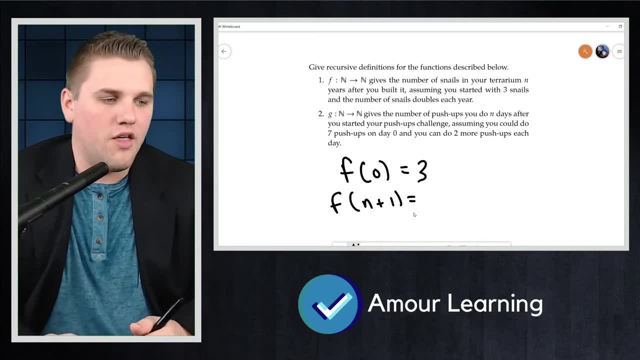 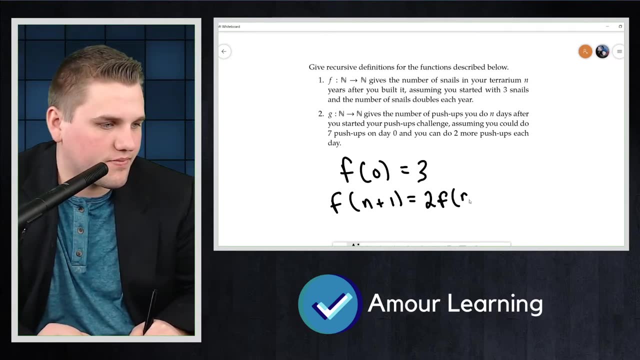 let's talk about f of n plus 1.. So if I want the next element of my function, the next input, then I have to take my previous input and I double it, So it'd be 2 times f of n. So, for example, if I want to know how many snails I'd 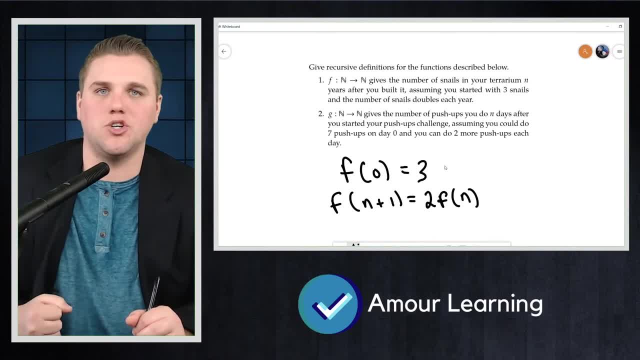 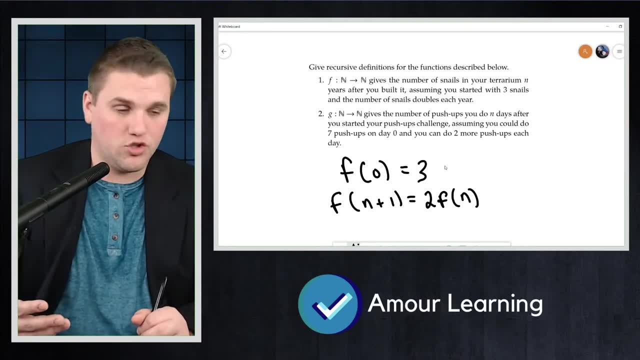 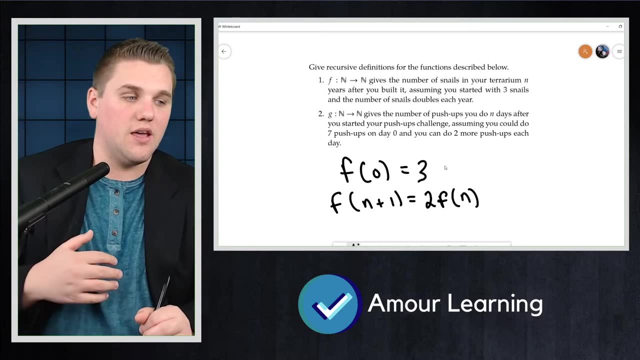 have after one year. I would take 3 and I would multiply it by 2.. Then I would take that element which is f of 1, which would be 6.. We would have 6 snails after one year. And to get to my next output, I would just plug in my 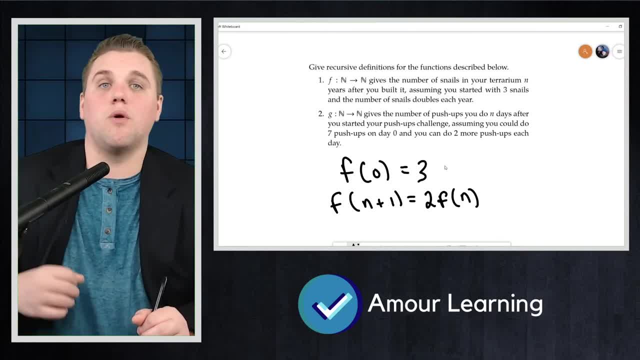 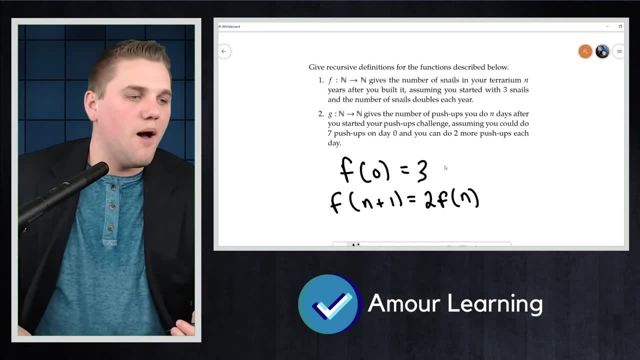 6 to get 12.. And then I would plug in 12 to get 24.. I can't do math in my head for some reason, But the idea is, this gives me a recurrence relation, namely that my f of n plus 1 is going to be f of n plus 1.. So if I want to take that, 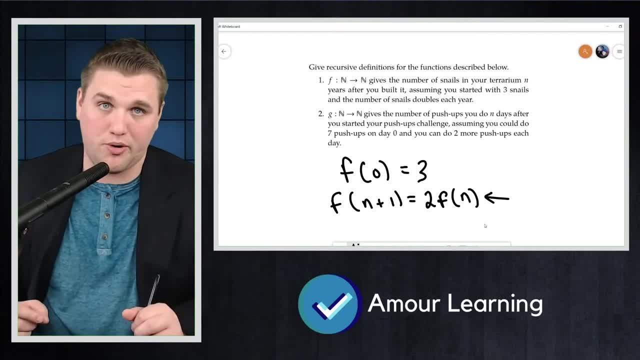 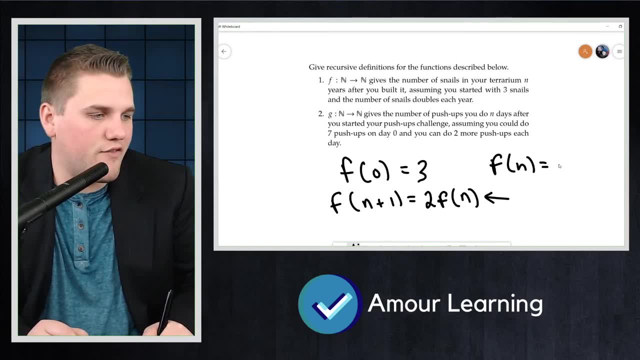 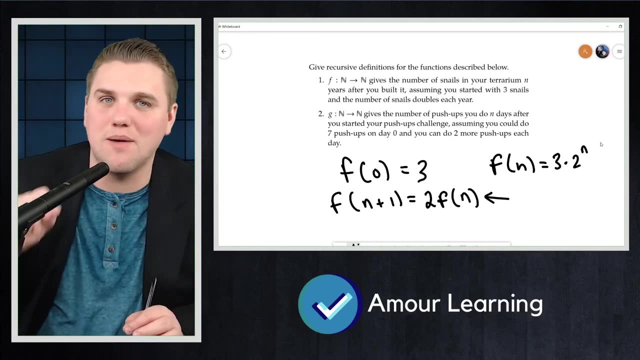 my next output is just 2 times my previous output. Now, technically you can create a closed form of this, namely that f of n equals 3 times 2 to the n, where you could just plug in n equals whatever you want and you can immediately find the. 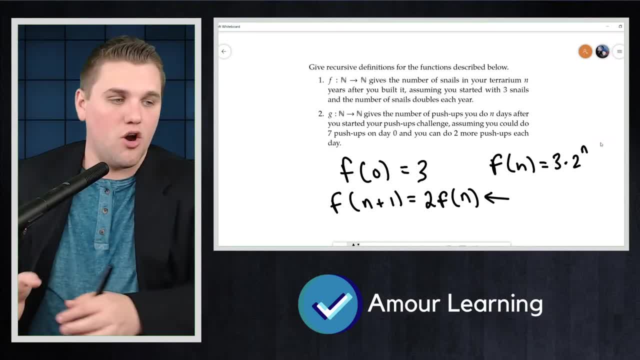 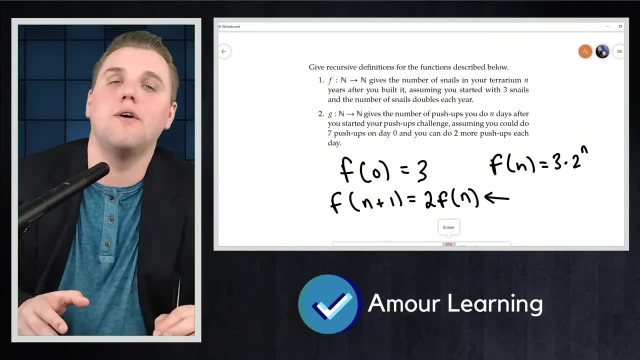 output. But that is different from a recurrence relation. Recurrence relation just tells you how do you get the next output And these functions are a lot easier to develop With real problems And again, this course is much more practical in my 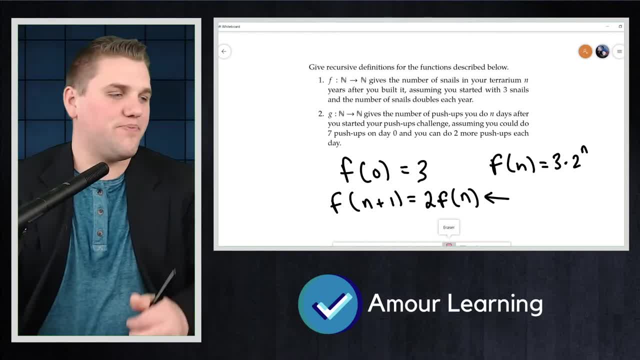 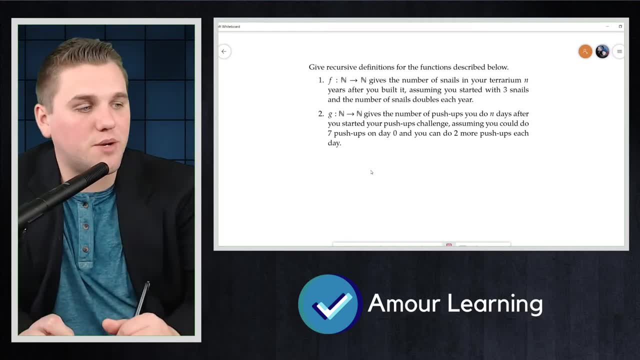 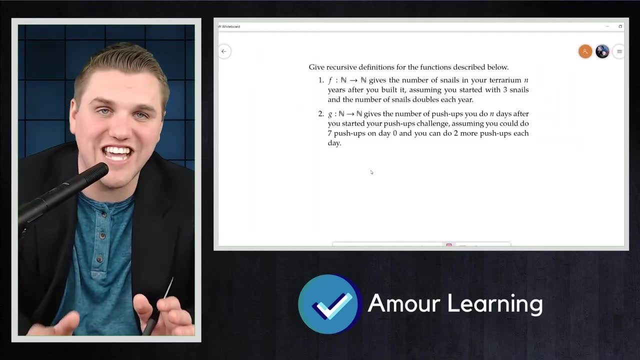 opinion, than other courses, including even calculus. All right, so let's do number 2.. G gives the number of push-ups you do and days after you started your push-ups. challenge assuming you could do 7 push-ups on day 0 and you could do: 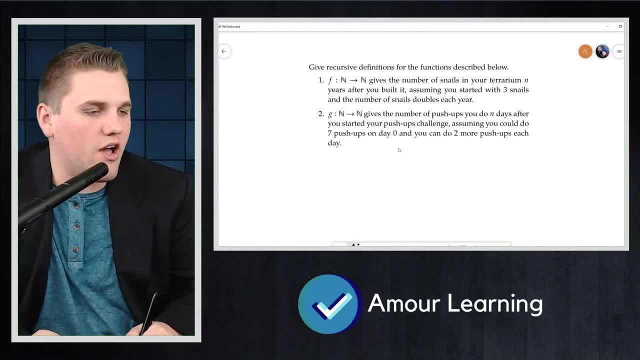 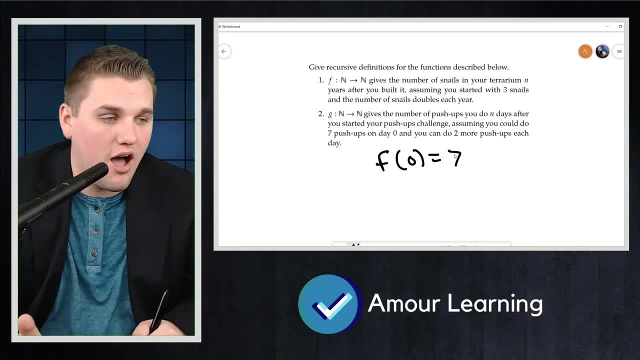 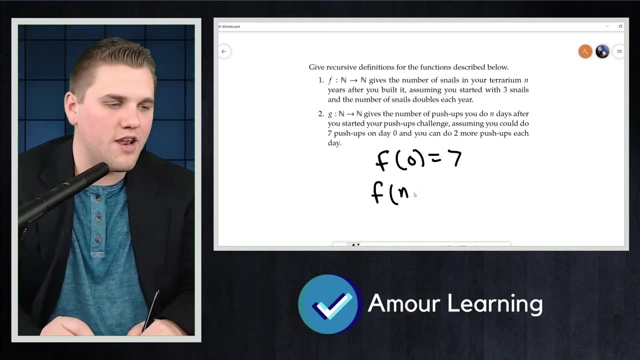 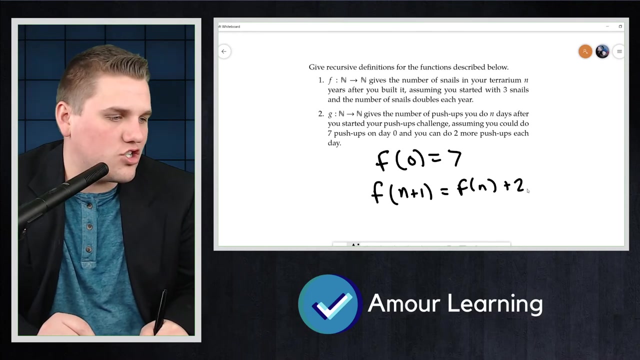 2 more push-ups each day. So in this scenario, my initial condition, which is 7, is 7.. I can do 7 push-ups after 0 days, But then to get my next day, the number of push-ups I can do on the next day, I just take the previous day and I add 2 more. 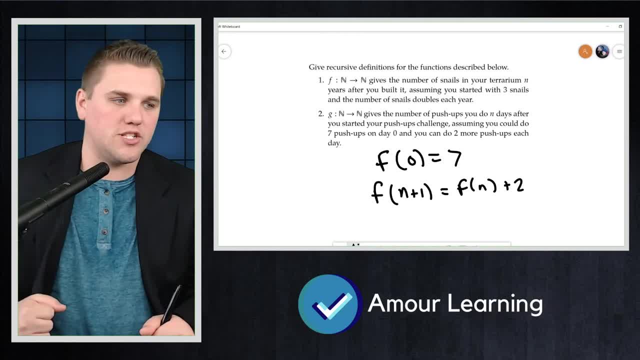 And so I just keep adding 2 to each output to get to the next output. So I start from 7 and then I add 2 to get to the next output, which is 9. And then I can do 11 push-ups. 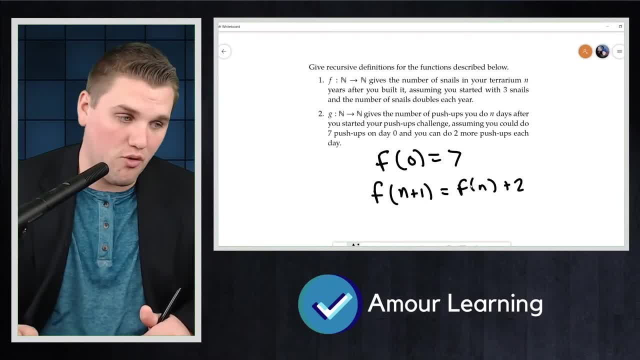 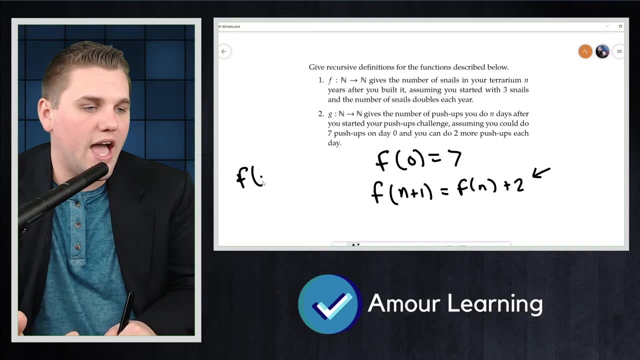 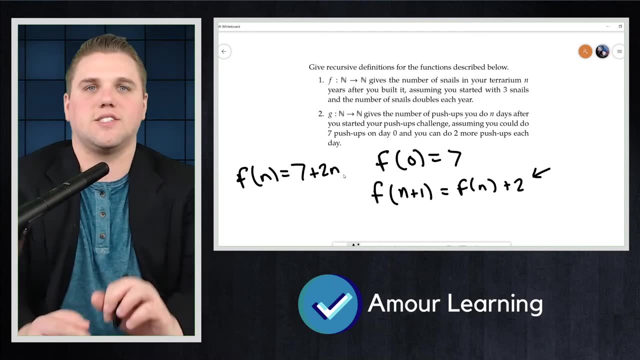 and then I can do 13 push-ups And I can do 15 and so forth. So this is my recurrence relation. Again, we could develop a closed formula: F of n equals 7 plus 2n. I believe would work Yes, And